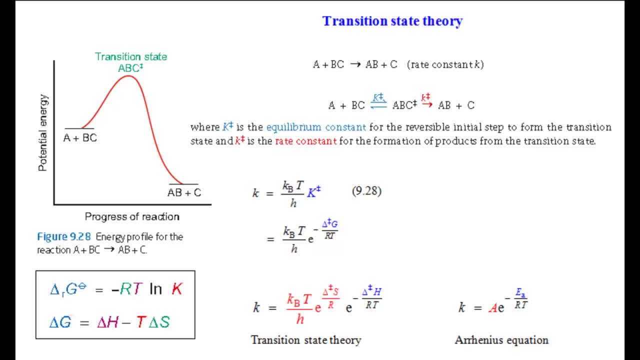 The transition state theory is based on a model of how a reaction takes place at a molecular level. Let's look at a general elementary reaction. A plus BC goes to AB plus C with a rate constant K. In the model, the reaction pathway from reactants to products passes through a transition state at the highest point on the energy profile. 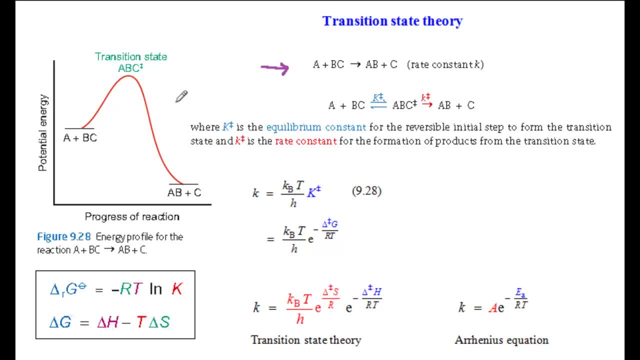 This is shown in figure 9.28.. The red curve shows the energy pathway from reactants to products. The transition state, ABC, is at the highest point on the pathway. Note the double dagger superscript which is used to label the transition state and also quantities involved in its formation. 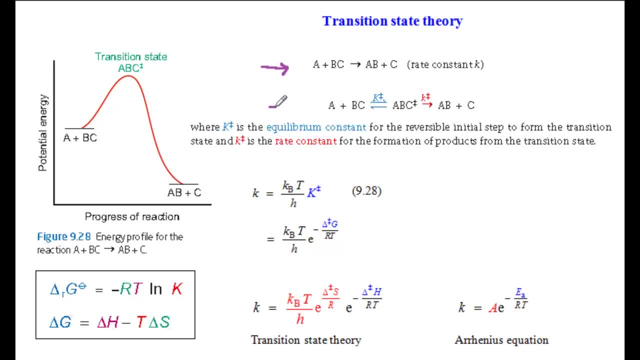 The third curve shows the energy pathway from reactants to products. The theory assumes that a pre-equilibrium is first established between the reactants and the transition state ABC, which then goes on to form the products. The large K double dagger in blue is the equilibrium constant for the pre-equilibrium forming the transition state. 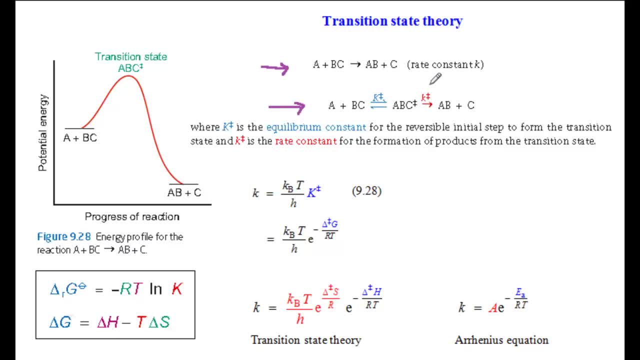 And the small K double dagger in red is the equilibrium constant for the pre-equilibrium forming the transition state. The third curve is the rate constant for the formation of products from the transition state. Now, using the ideas developed in section 9.6 for this type of reaction mechanism involving a pre-equilibrium, 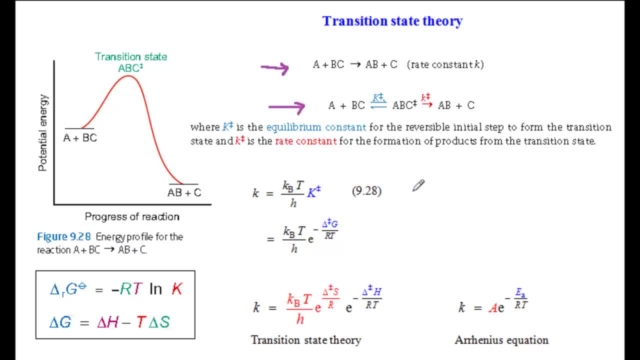 it is possible to obtain an expression for the overall rate constant K in terms of the equilibrium constant K double dagger and the temperature constant and the temperature T. This term is constant, Kb is the Boltzmann constant and H the Planck constant. 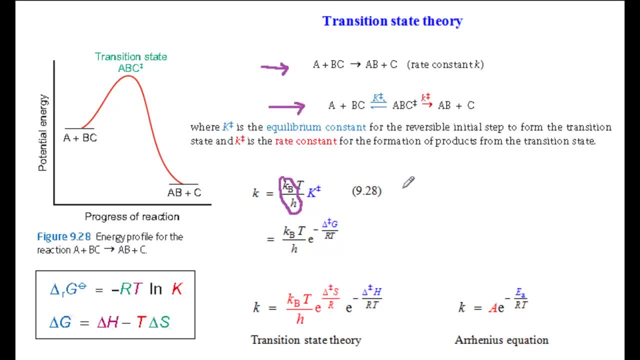 Don't worry about the derivation and the maths at this stage. The important point to note is that this equation links the rate constant for the overall reaction with the equilibrium constant for the formation of the transition state. Now you need to use some thermodynamics from chapters. 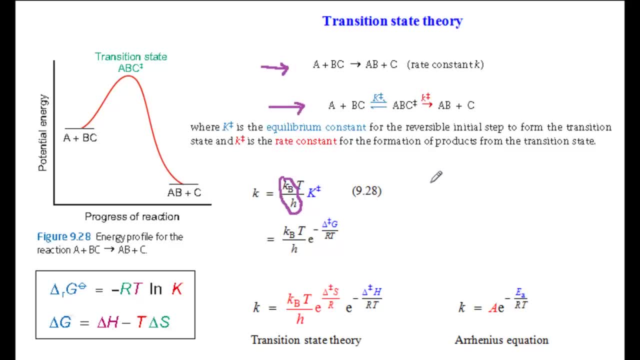 14 and 15, because K double dagger is related to other thermodynamic functions involved in the formation of the transition state. This is equation 15.4, which links an equilibrium constant K with the standard Gibbs energy change for the reaction. It can be rewritten in this form: 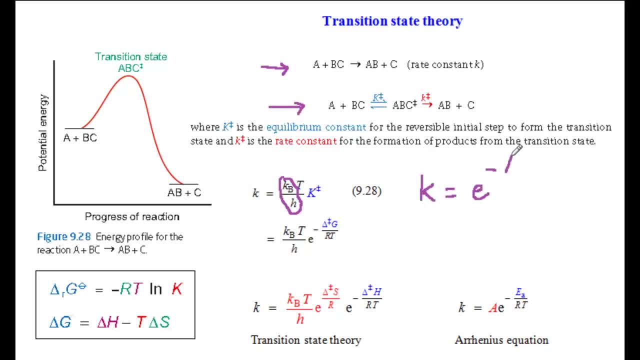 Equilibrium constant equals E to the minus delta G standard over RT. So you can substitute for K double dagger in equation 9.28 to give this expression here, where delta G double dagger is the Gibbs energy change, And since delta G equals delta H minus T delta S, 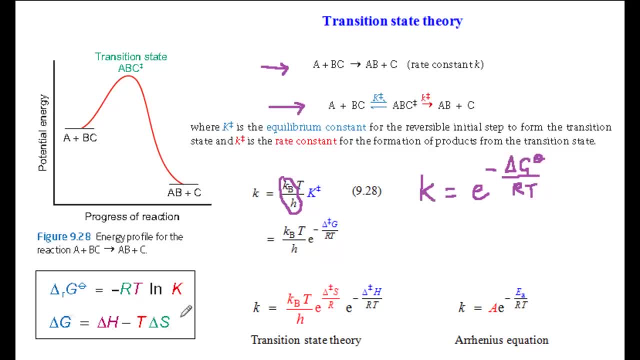 equation 9.28 can be rewritten yet again into this form here, where delta H, double dagger, is the enthalpy of activation and delta S is the energy change for the formation of the transition state from the reactants. So this is the Gibbs energy of activation. 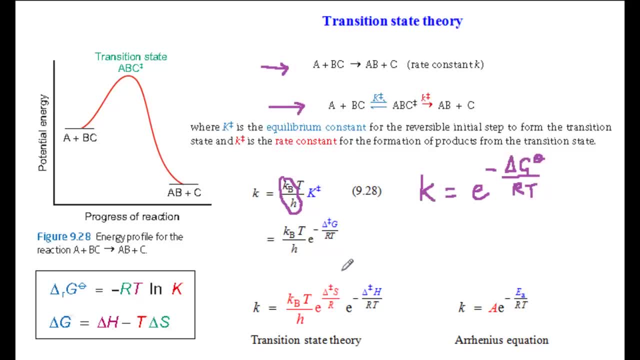 Delta S double dagger is the entropy of activation. Now compare this equation with the Arrhenius equation from section 9.7, which shows the effect of temperature on the rate constant. Remember the equation on the left is derived mathematically from a theoretical model. 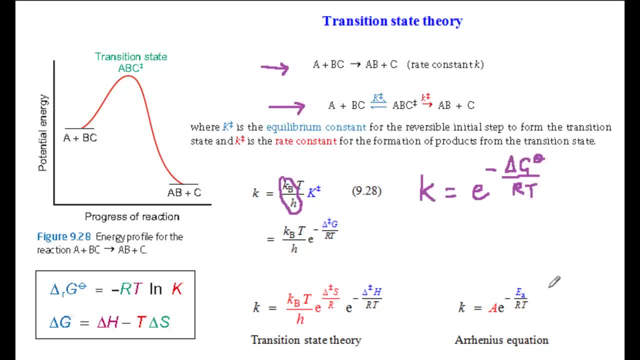 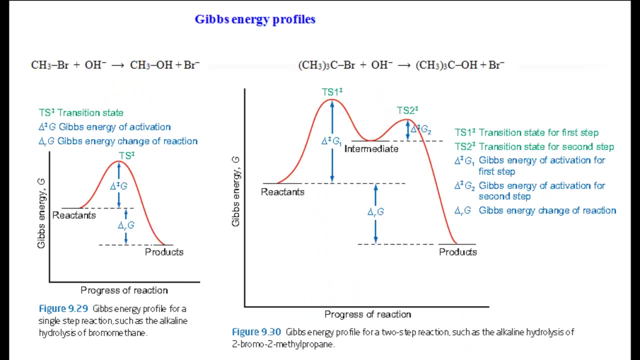 whereas the Arrhenius equation on the right represents experimental observations. The enthalpy of activation, delta H double dagger- corresponds to Ea, the activation energy And the term in red, which contains the entropy of activation, corresponds to A, the A factor in the Arrhenius equation. 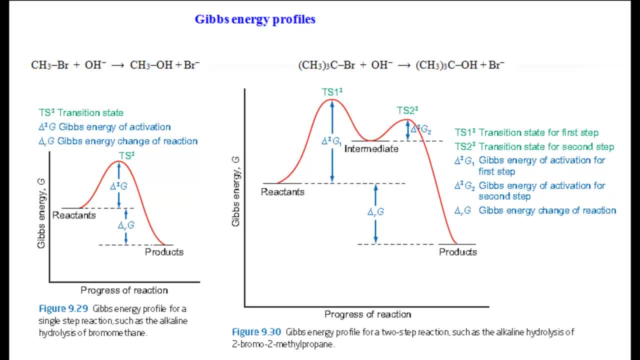 A useful Things. A useful Things. way to follow the progress of a reaction is to plot the Gibbs energy G as the reaction takes place. This is called a Gibbs energy profile. We've seen that the transition state theory links the Gibbs energy of activation directly to the rate. 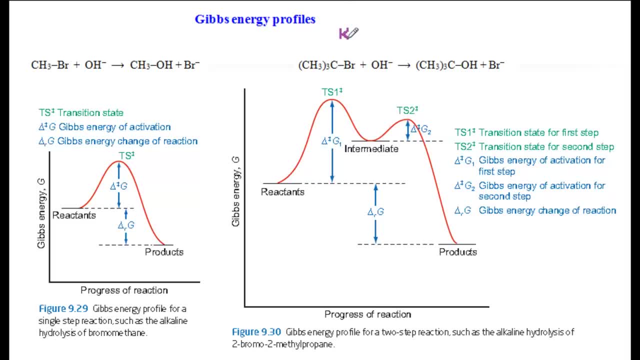 constant K for the reaction. K the rate constant is proportional to E to the minus delta G double dagger over RT. So the greater the value of delta G double dagger, the smaller the value of K the rate constant and the slower the reaction. 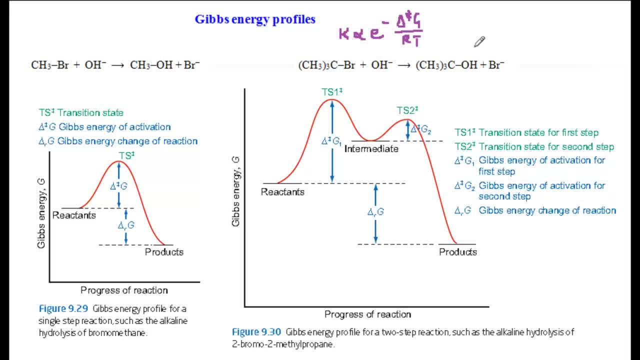 Also, the Gibbs energy change incorporates both an enthalpy term and an entropy term, which can be very important. For these reasons, Gibbs energy profiles, rather than enthalpy profiles, are used extensively in organic chemistry and in biochemistry to illustrate the mechanisms of reactions. 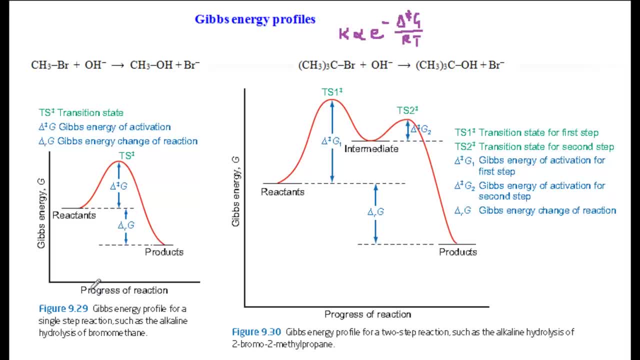 Figure 9.29 shows the Gibbs energy profile for a concerted single step reaction such as the alkaline hydrolysis of a primary halogen alkane such as bromomethane, which takes place by SN2 mechanism and is an elementary reaction. 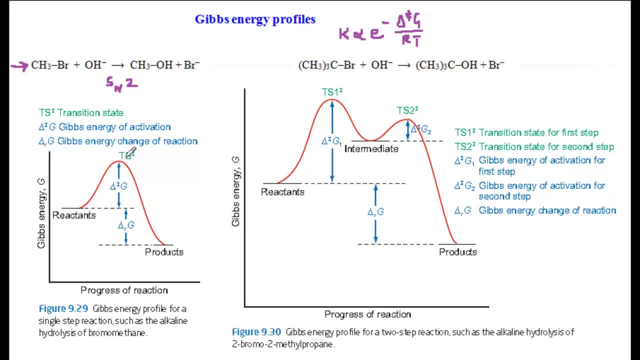 There's a single maximum corresponding to the transition state for the reaction Delta G. double dagger is the Gibbs energy change for the formation of the transition state. 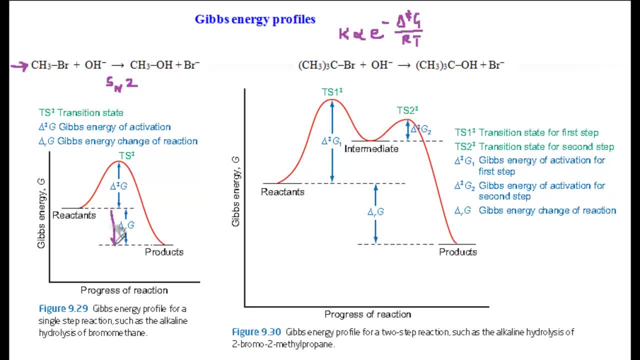 confuse this with delta gr, which is the gibbs energy change for the reaction and is the difference in gibbs energy between the reactants and the products. figure 9.30 shows the gibbs energy profile for a complex reaction.